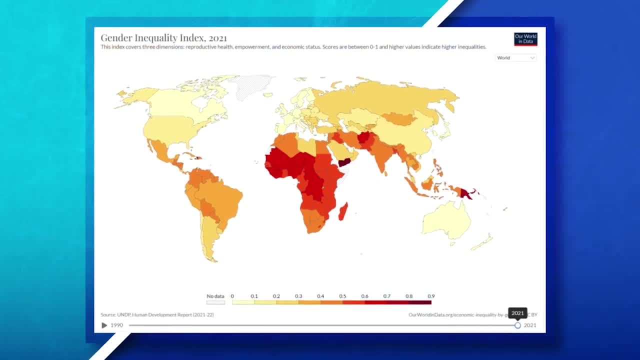 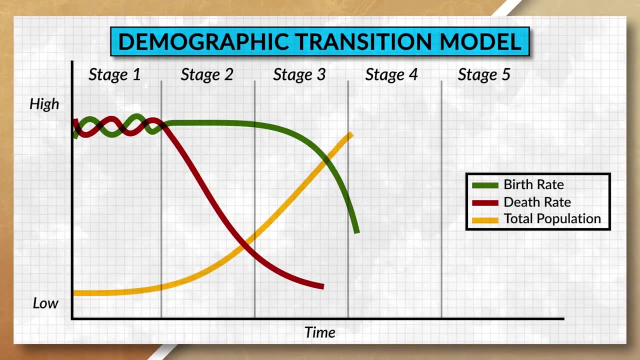 around the world are gaining more economic, political and social opportunities. As countries continue to develop and advance in the demographic transition model, women start to gain more opportunities in society. However, countries that lag behind in the demographic transition model are the ones that are going to have to face more challenges. 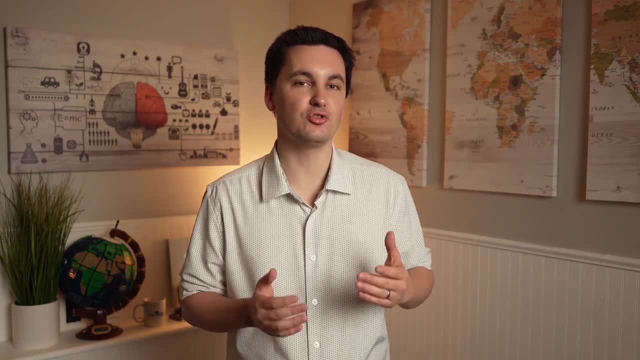 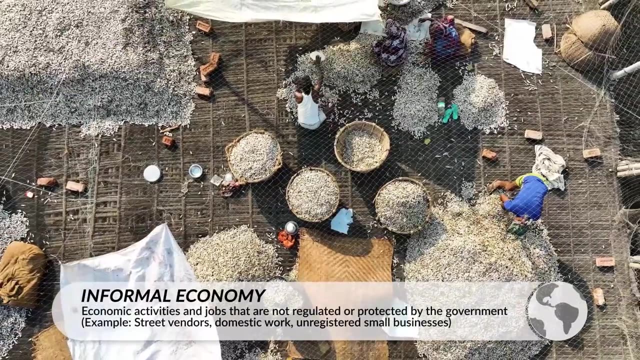 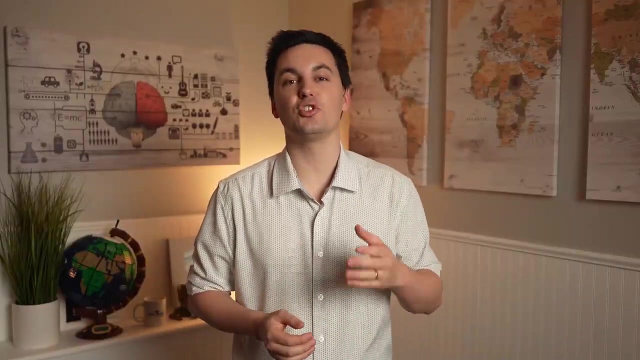 Women in their economic development often tend to have more traditional gender roles in place, which often places women in roles that are part of the informal economy. The informal economy consists of jobs that are not regulated or monitored by the government. To better understand the development of a society and to gain insight into women and the opportunities that exist in. 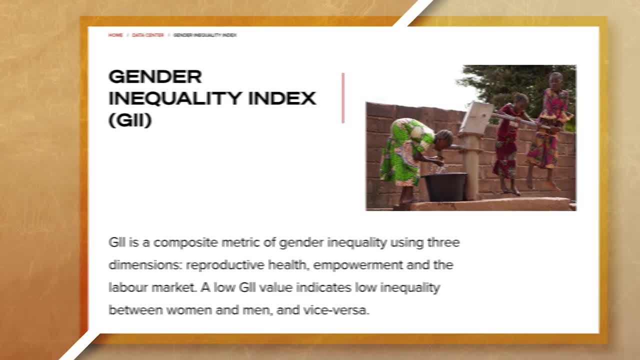 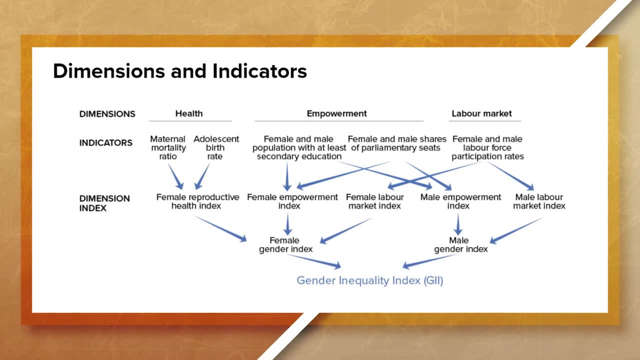 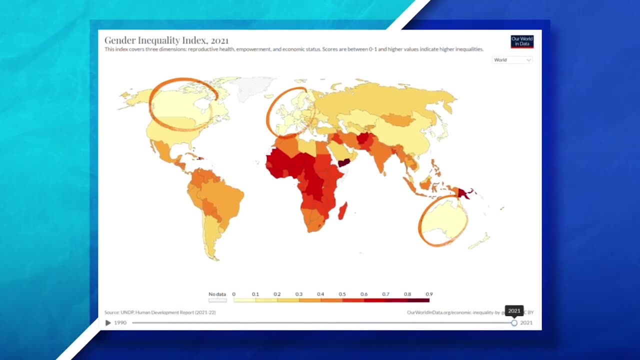 society for them. we can look at the Gender Inequality Index. This index measures reproductive health, empowerment and labor market participation to illustrate the amount of inequality and equality in a country. Countries that have a lower GII have less inequality between genders in society, and countries that have a higher GII have more. 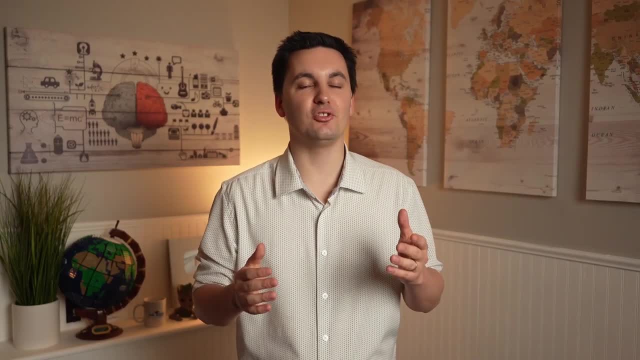 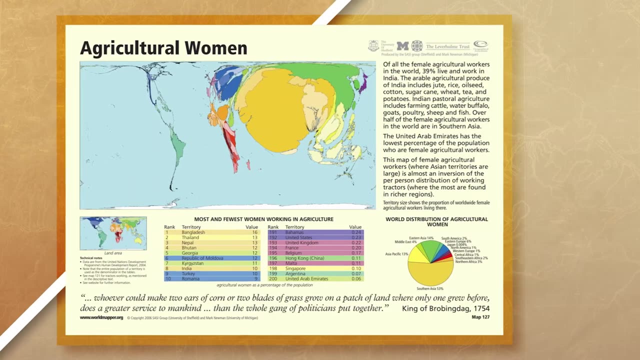 inequality between the different genders Today. if we look at regions such as Southwest Asia or Sub-Saharan Africa, we can still see inequality between genders and see that women often still make up a large percentage of the agricultural workforce. Countries that are less economically. 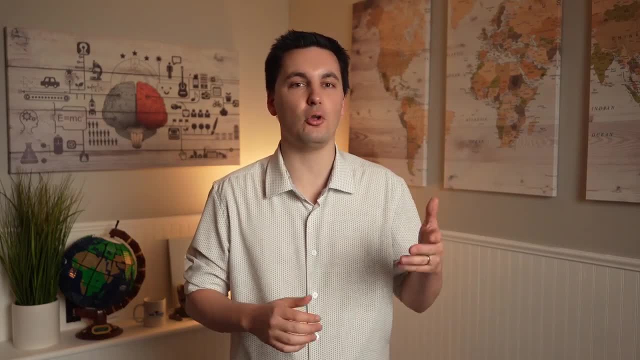 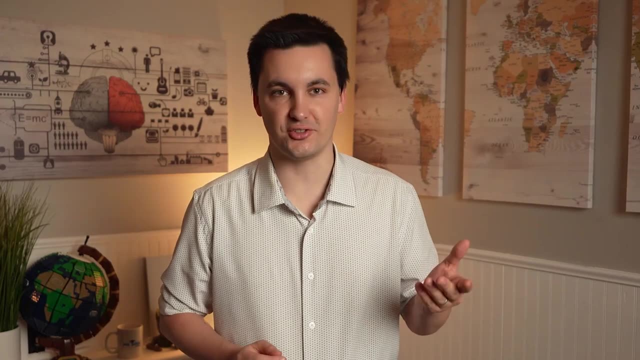 developed traditionally tend to have more traditional gender roles. So if we look at the gender roles for women, we can see that women often have more traditional cultural norms and gender roles for women. These roles often have been in place for many years and are well established in. 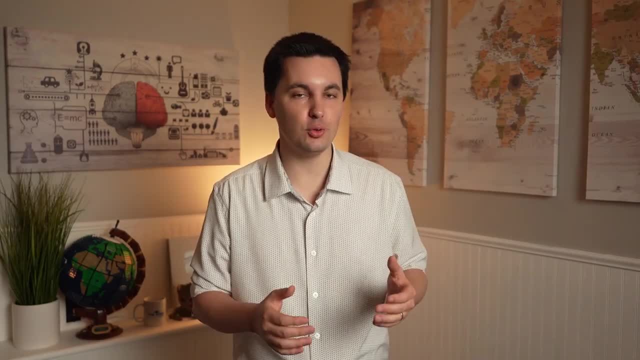 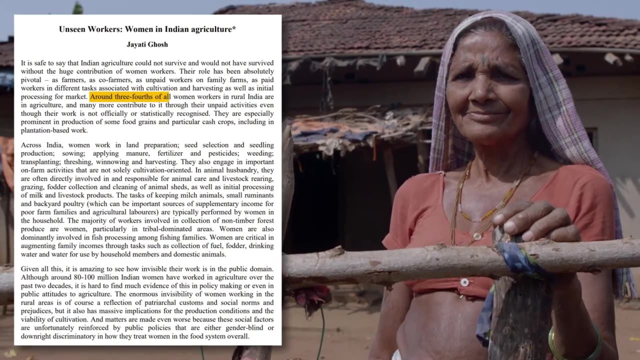 society. Oftentimes, these cultural norms will limit the opportunities that different individuals in a country have. We can see this noted, for example, in India, where around three-fourths of all women workers in rural India are in agriculture, and many more contribute to it through their 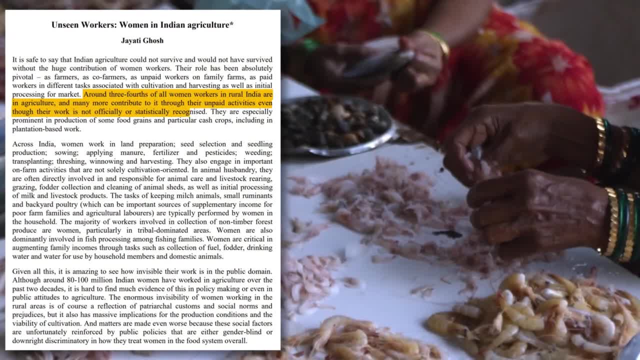 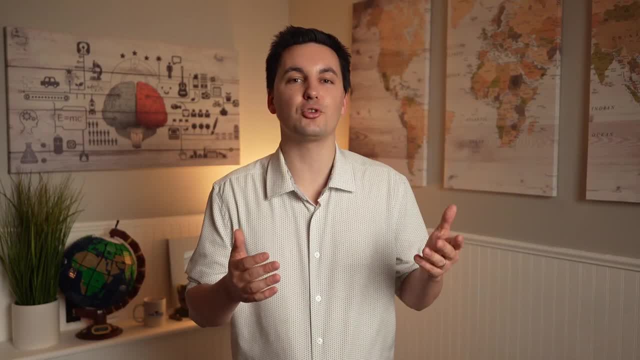 unpaid activity, even though their work is not officially or statistically recognized. Now, as countries develop and move further down the line, the gender roles for women are more important. They start to allow more opportunities for women in society. Society also starts to see. 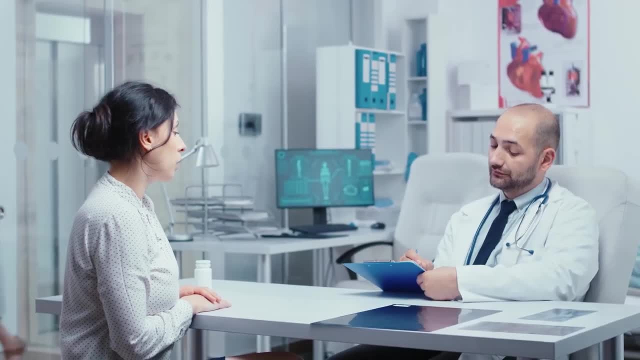 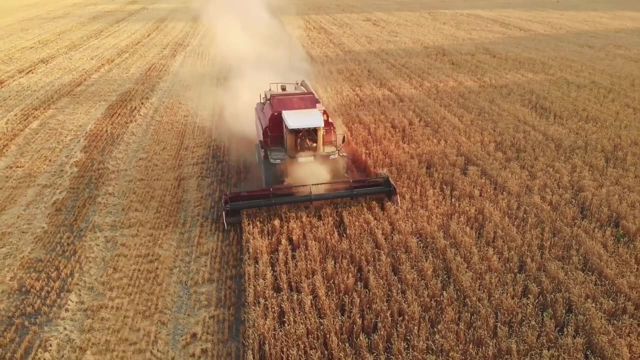 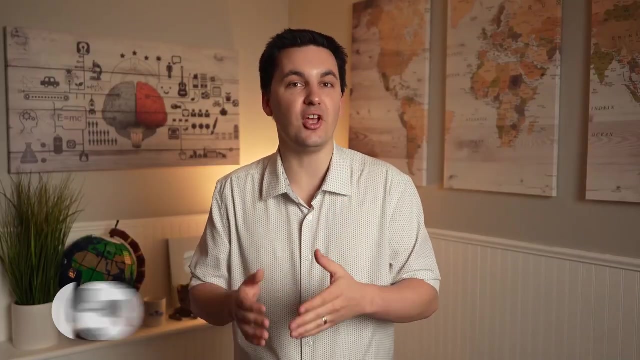 changes in the production of goods and services, since more people have access to money and capital. As society develops and changes, agricultural production shifts as well. Farms start to utilize new machinery, which reduces the amount of human labor needed for production, thus resulting in a lower agricultural density for society. Economic growth also leads to increased rates of urbanization, as well as the increase in the number of people who live in rural areas. So, if we look at the demographic transition model, they start to allow more opportunities for women in society. Society also starts to see changes in the production of goods and services, since more people 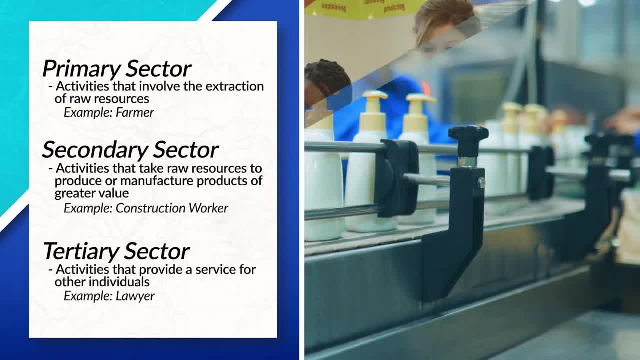 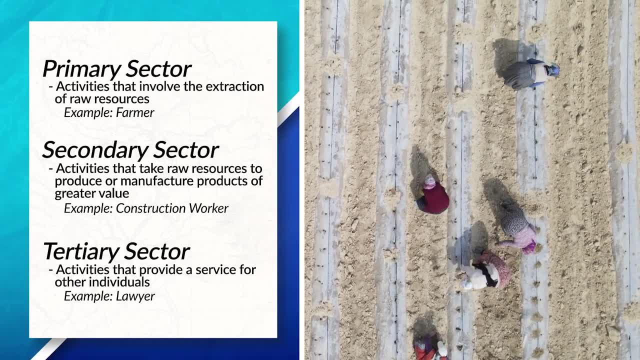 have access to money and capital As more jobs open up in the secondary sector and the tertiary sector, which allow citizens to participate in new ways in the economy. But even with all of these changes, we still often see women working with agricultural products. 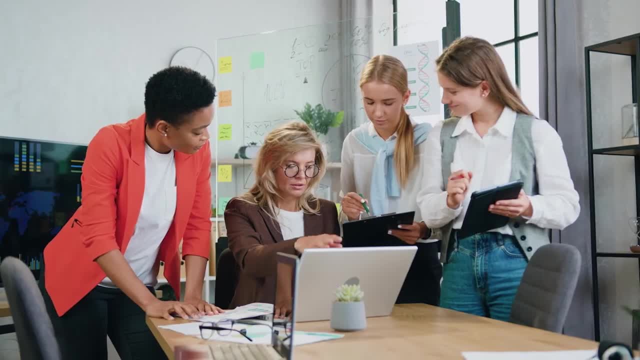 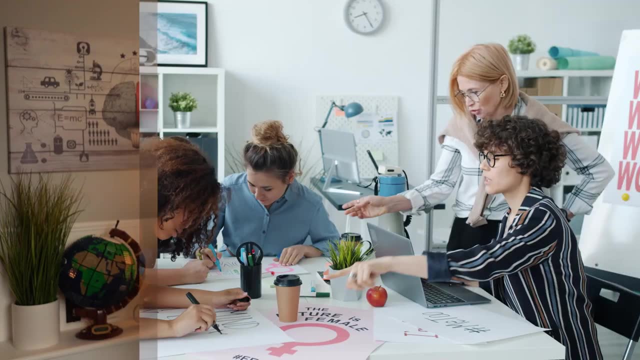 and in industries with lower-paying jobs. Now, as society continues to develop, we continue to see more and more opportunities for women. However, many traditional gender roles and stigmas still linger. Women are still pushing for equal representation and opportunities in the workforce. 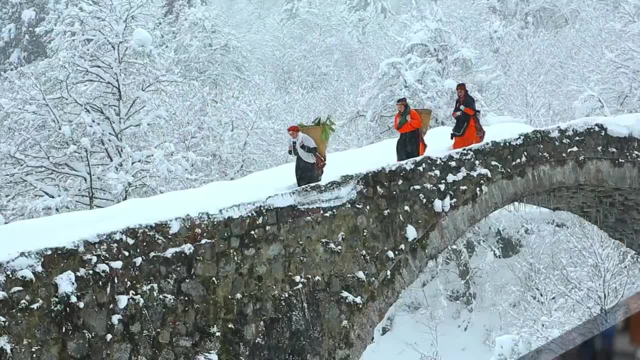 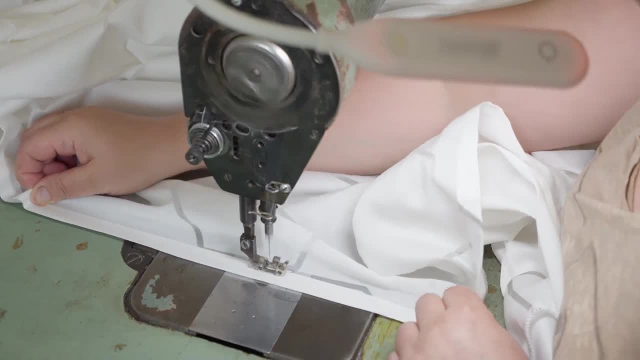 political offices and their own social and economic opportunities. However, there are also opportunities for women in their own communities. Unfortunately, today we can see that many less economically developed countries around the world still have women in the informal economy with little political and social protection. Today, women in less economically 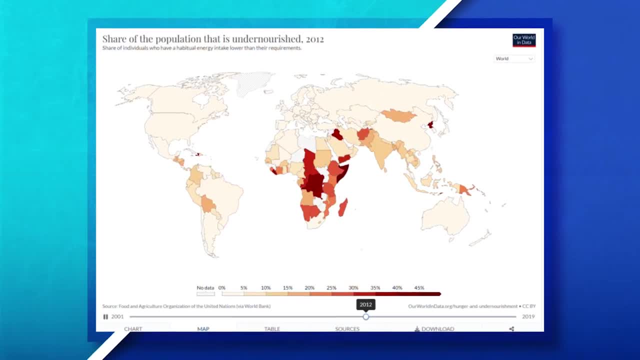 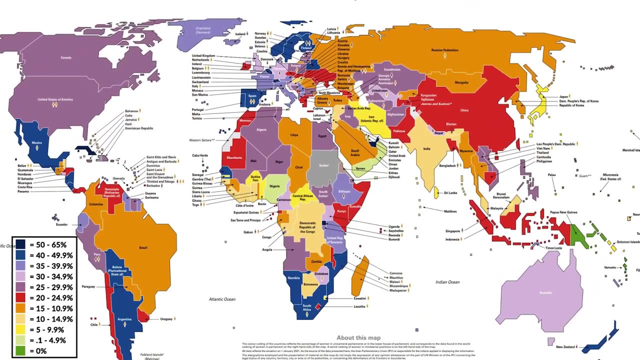 developed countries are also more likely to be malnourished, as caloric intake is often prioritized for the men. Women in these areas are also less likely to have political representation and may not even be able to own land. But as countries develop both economically and socially, we start to see. 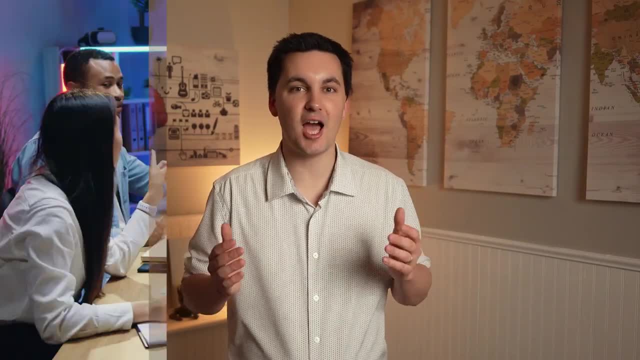 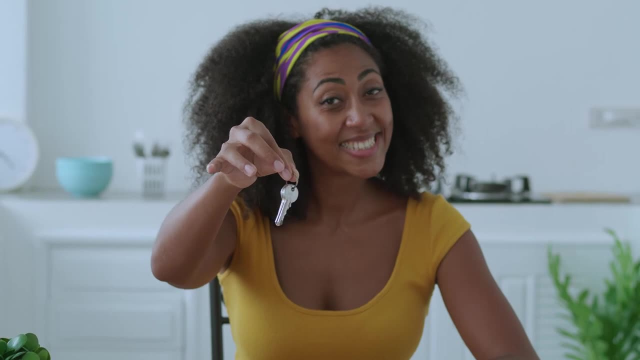 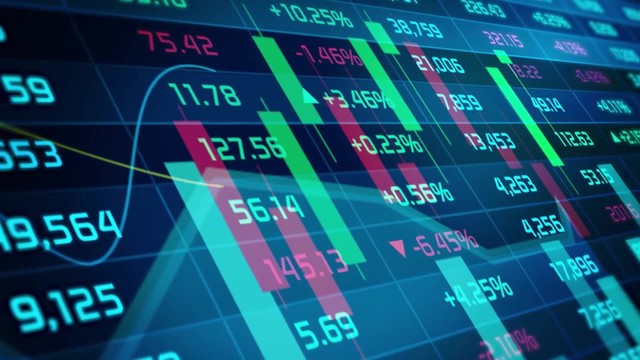 women gain political and social opportunities in society, be able to participate more in the formal economy, gain different legal protections and see land ownership for women increase. Plus, when countries allow women to have a more active role in society, they tend to see higher economic growth and a higher standard of living for all people in the 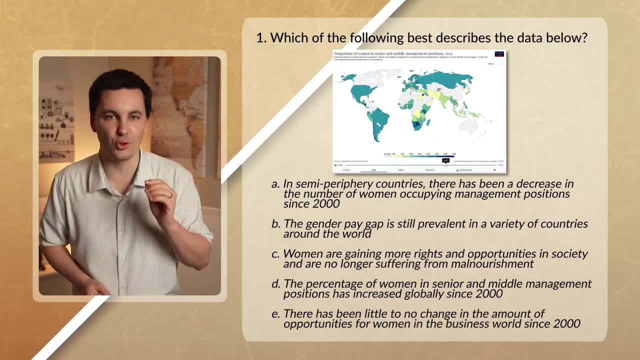 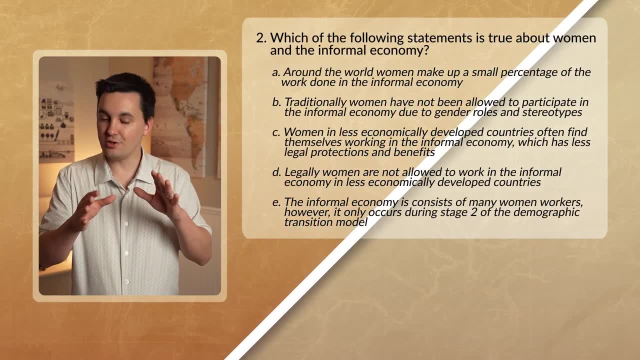 society. Alright, geographers, now comes the time to practice what we have learned. When you are done, don't forget to head over to my Ultimate Review Packet and check out the Unit 5 Summer Story video Again. you'll also find exclusive videos to help you with your AP Human Geography. 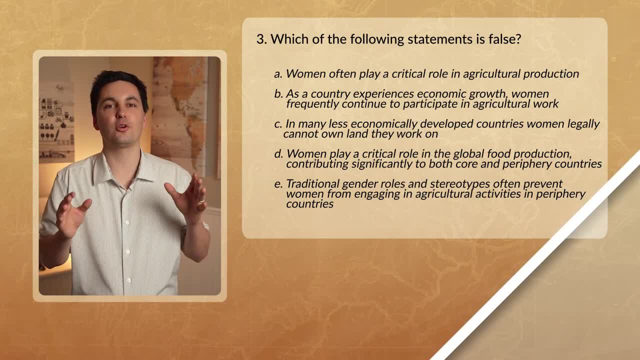 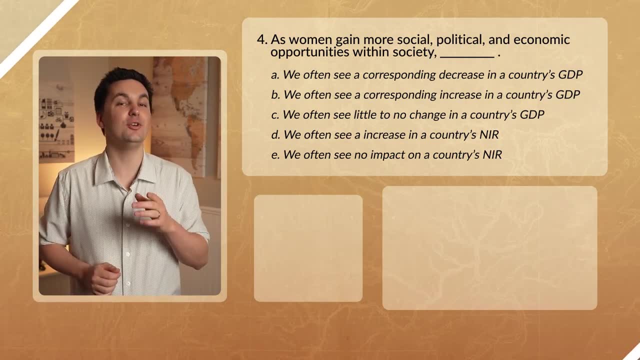 studies, review packets, practice quizzes and all the other resources for each unit of AP Human Geography. Thank you so much for watching this video. As always, I'm Mr Cyn and I'll see you next time online.